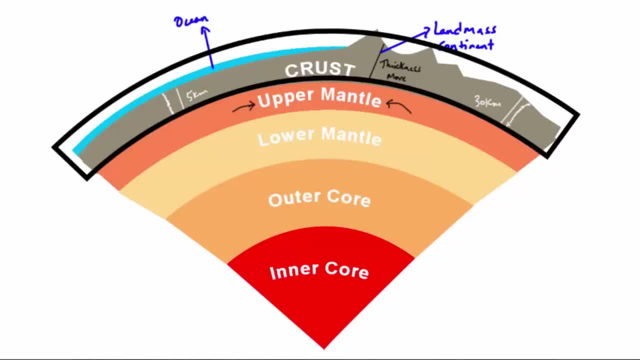 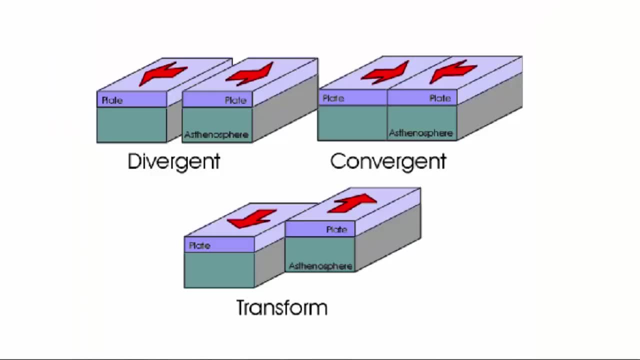 Earth, in that we clearly understood that the crust is divided in the form of some major and minor plates, And these plates have three types of motions. When two plates come towards each other, we call that as convergent boundary. When they move apart from each other, we call 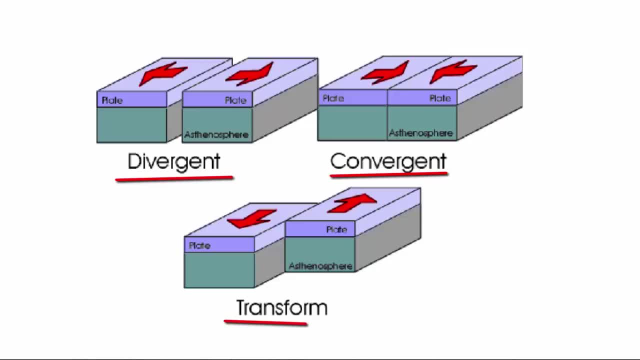 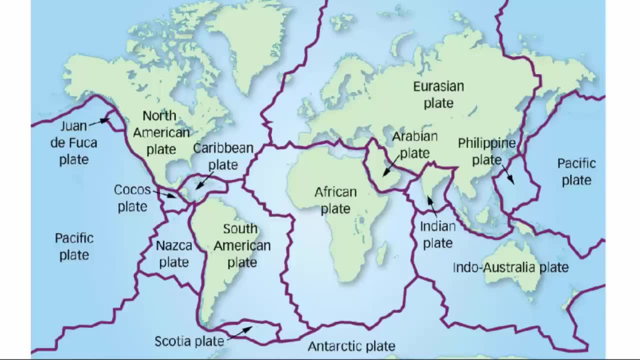 that as divergent boundary, And then sometimes these plates slide past each other. So it is because of these three movements you will see changes on surface of the earth, ie the crust. Now mountains emerge because of this, Then we have faults, huge cracks on. 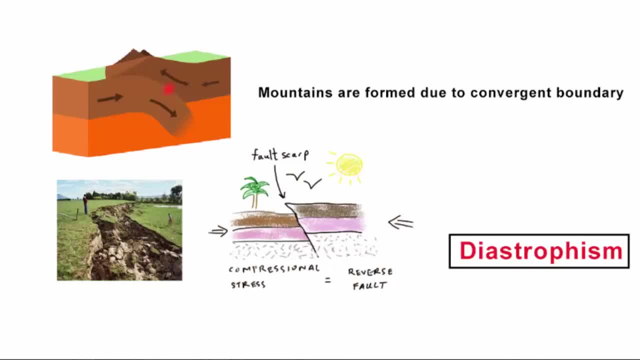 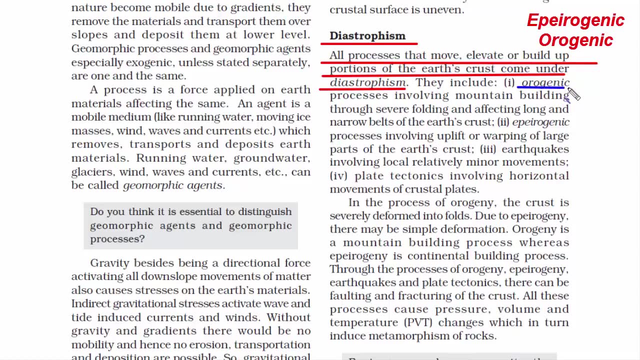 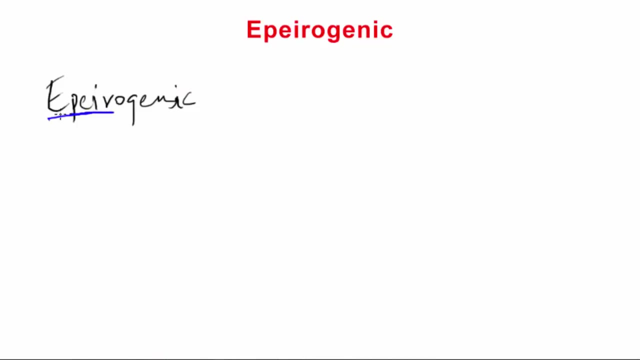 the land surface because of this. So this is what is diastrophism. Now, diastrophism is broadly classified into two types, ie epirogenic movement and orogenic movement. The first one is epirogenic movement. The word epirogenic, let's break the word. 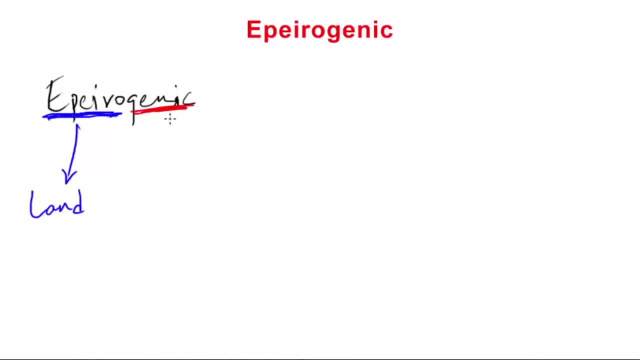 The meaning of the word epiros is land and genic can be derived from genesis, which means birth or origin. So together, epirogenic means the origin of land. Epirogenic movements are vertical, So to make a piece of land, all the materials. 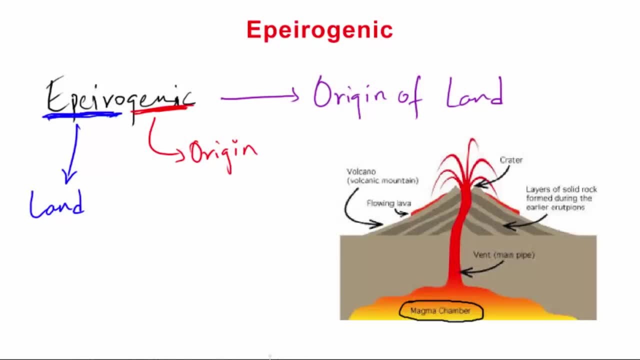 come out from within the earth's mantle, ie the magma. When that solidifies, it becomes hard rock, and once rock begins to break down through weathering, it turns into sediments and that becomes land for us. So the movement is vertical. Now what happens in orogenic? 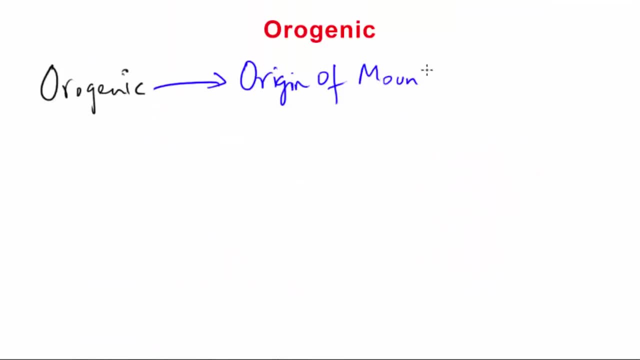 movements is that orogeny is the origin of mountains, So their movements are sideways or horizontal movement. Now, what happens when crustal plates move horizontally? They either slide or slide past each other. But then in this we know it's a mountain forming process. 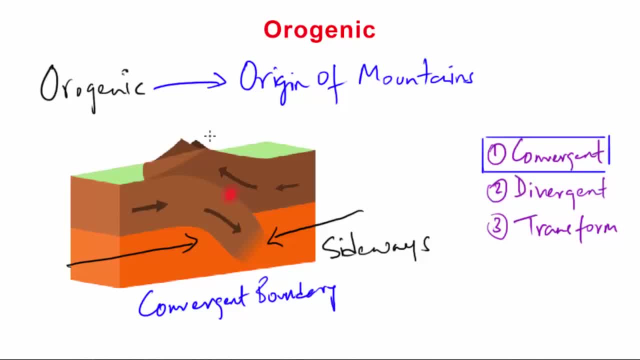 And mountains are only possible if two crustal plates come closer. When two plates come closer, the smaller plate goes under the bigger one. That causes larger piece of rocks to twist and fold, making the land surface to elevate, And that forms a mountain. Now let me show. 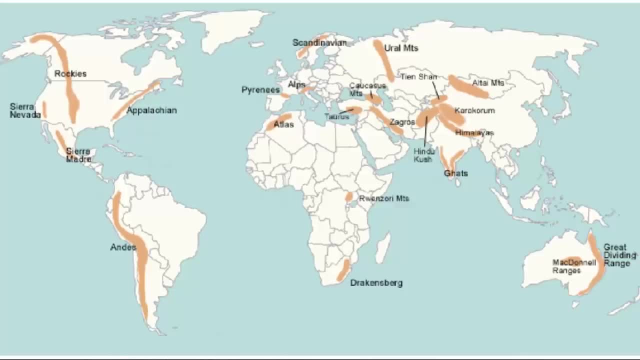 few places of earth where this kind of mountain building processes took place. You will find these places Here. we have the Andes, Then here is Himalayas, Then here is Ural Mountains. This part is known as Rocky Mountains of Western United States, So always remember orogenic.